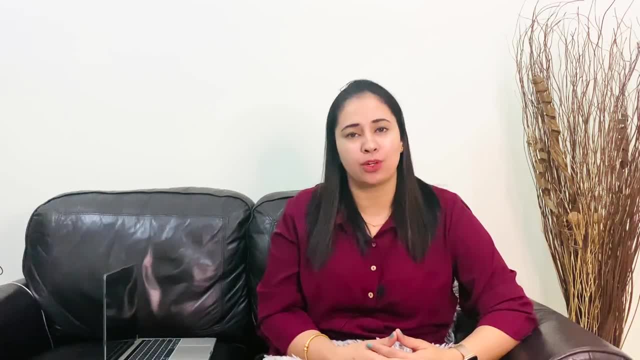 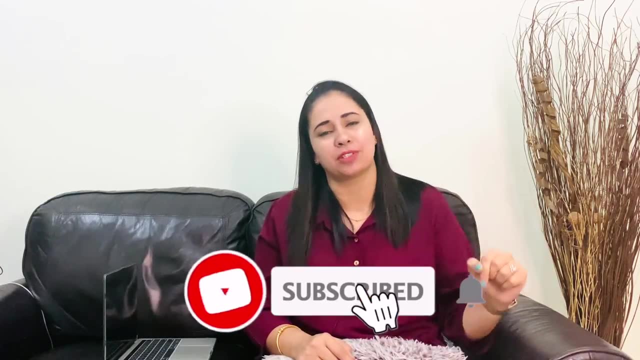 I think you will be able to answer most of the questions which the recruiter is going to ask in a primary teacher interview. So let's start today's video. If you are new to the channel, do consider subscribing and press the bell icon, And if you are a return viewer, thank you so much. 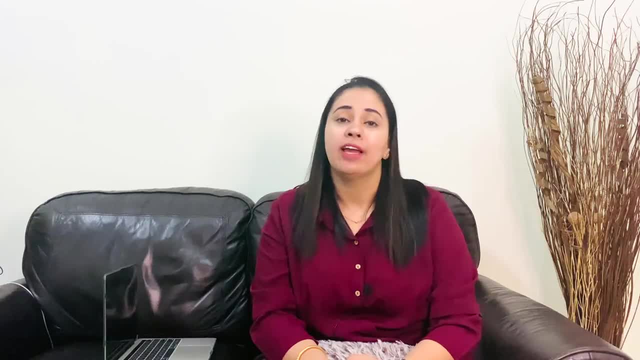 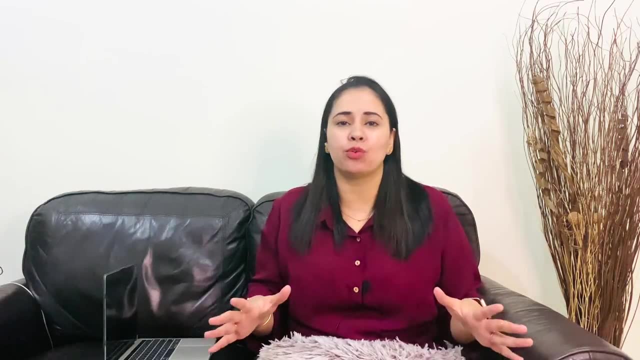 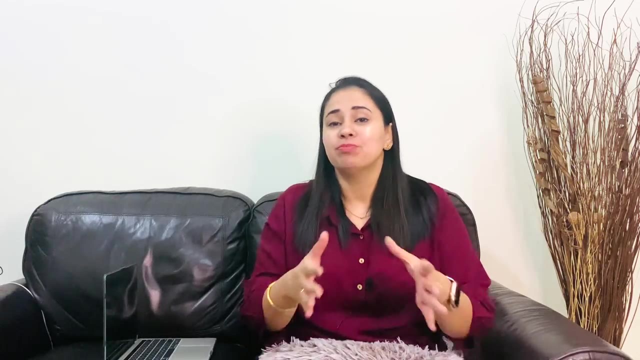 for supporting us. I hope I am adding value to your life, new skills to your profession. So let's start today's video. So the first question is which every recruiter will ask: tell me about yourself and why you want to become a primary school teacher. See the. tell me about. 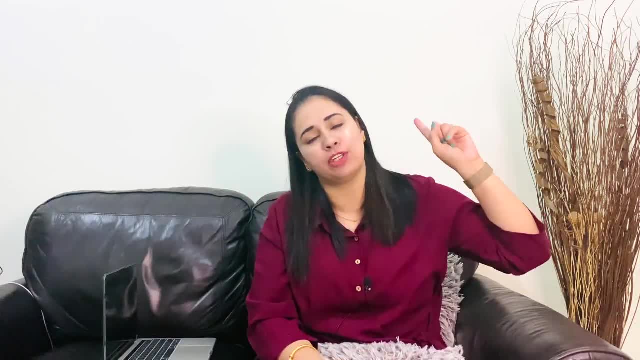 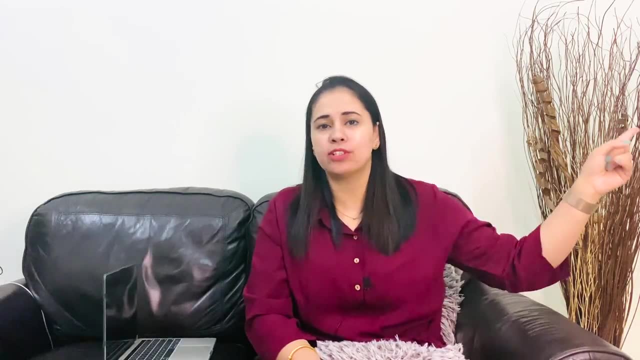 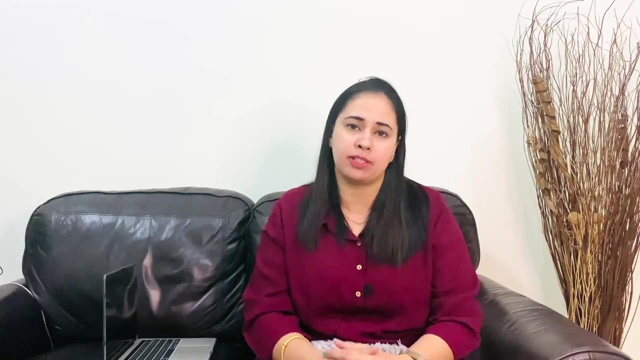 yourself is such an important question that I made a separate video about that question only. So first you post this video and go and check out that link above and watch that video and then come back and continue with this question. Now the second part of the question is why you want to become a primary. 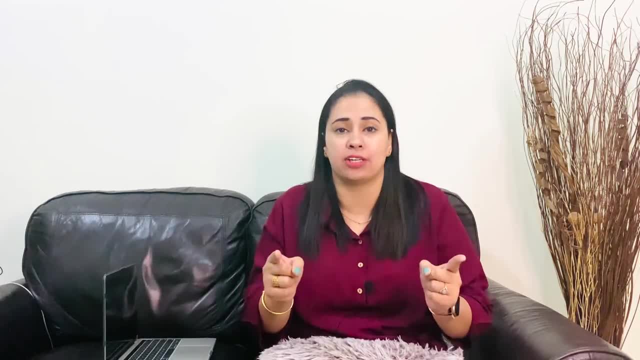 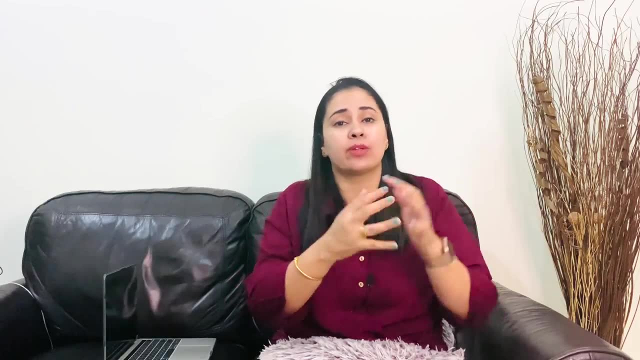 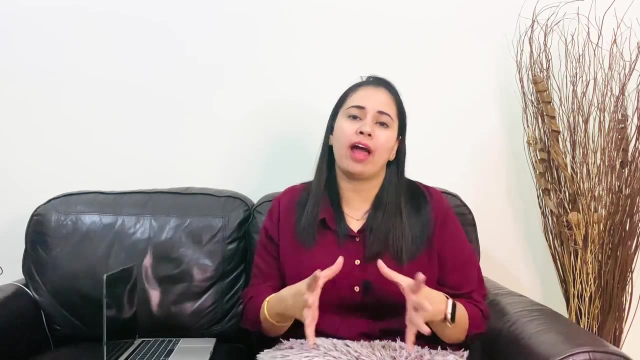 school teacher For that question. you need to show your passion, You need to show him why you have chosen this profession, how you are, like you know, connected with the children, So you can say that when I was doing my BA, at that time I got placed in a school where I was teaching. 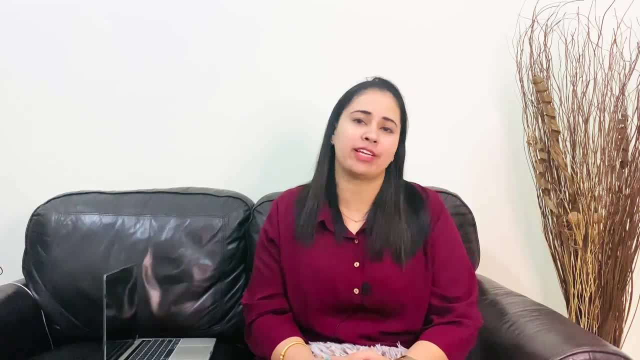 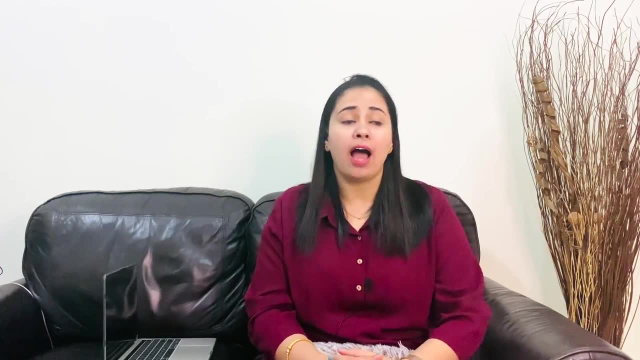 grade, whatever grade you are going to apply for. For example, where I was teaching grade one to two and I really get attached with some students, I was really feeling passionate when I was solving their queries, when I was answering their questions, and I really enjoy working with them. 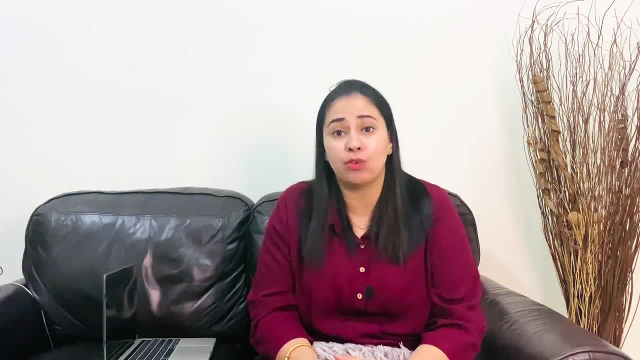 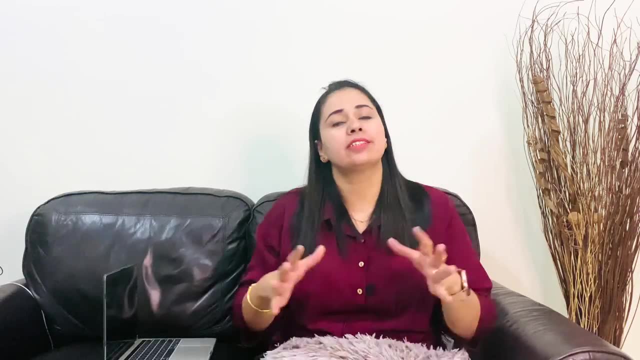 teaching them. So that's how you will show your passion and you will answer the question that you are really want to be in this profession and you really want to be with the children. So the second question is: tell me, is there is not this job very challenging, especially being a primary? 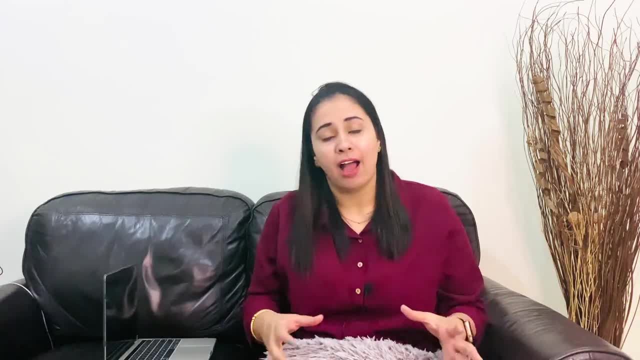 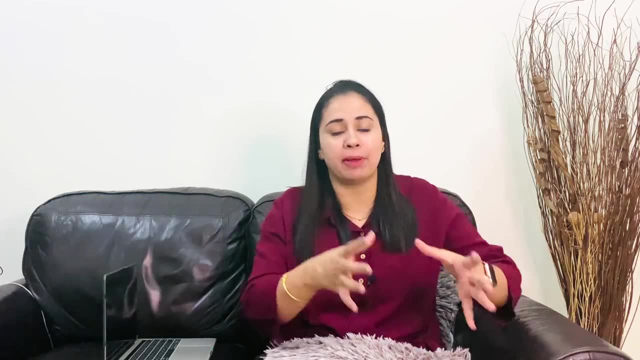 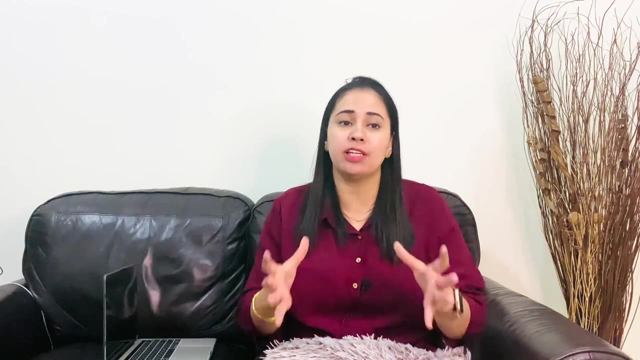 teacher with the small children. Yes, absolutely. I found this job very challenging, especially being the responsibility, because we are responsible to shape and to mold the lives. We are putting a basic stone which turn into a building, So we have the responsibility to put that basic stone properly. 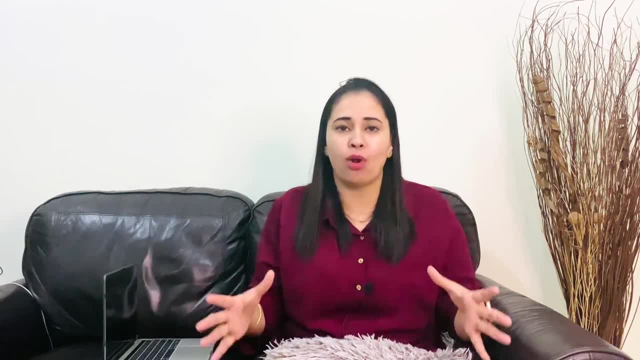 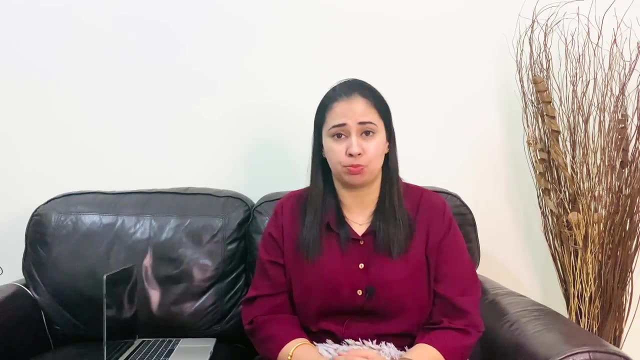 so that the building will stand on that for a long time. So I think that's the first question. The second question is to think of your future project. If you think that you are going to be a primary teacher, then I think that you can be a primary teacher in the first year of your 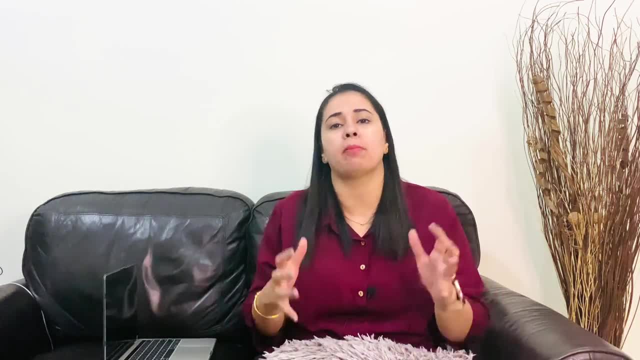 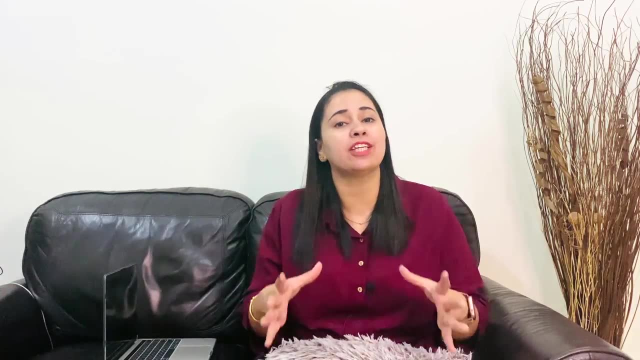 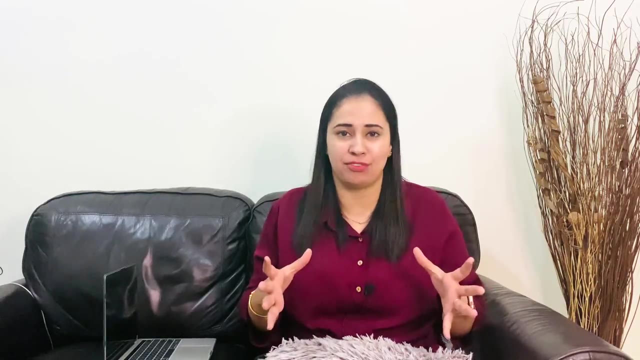 degree. But the right question is to think like a parent who is going to take care of their kids for a long time and with a good infrastructure. So I really mean it And I'm ready for this responsibility. Question number three: how you manage naughty children especially. 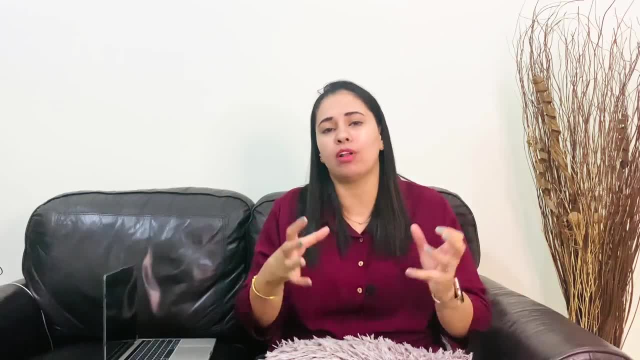 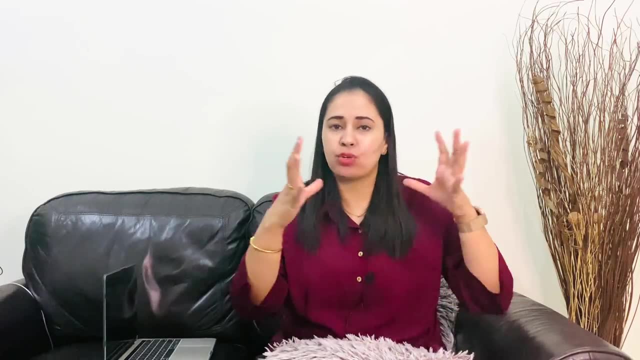 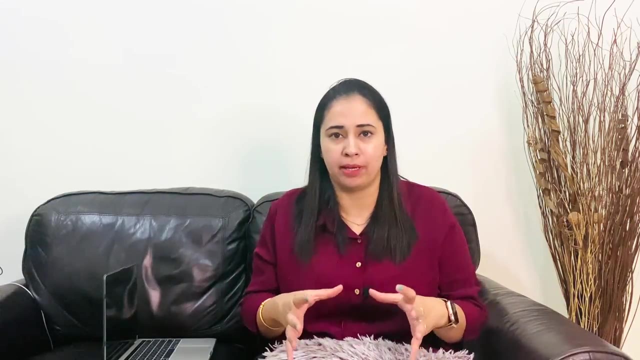 the maximum i can. i will try to involve the latest technology. i will include the games, the hand-on activities. i will try to use the smart board as much i can and i will try to bring their interest into the particular topic so that they will forget about the other games, other naughtiness. 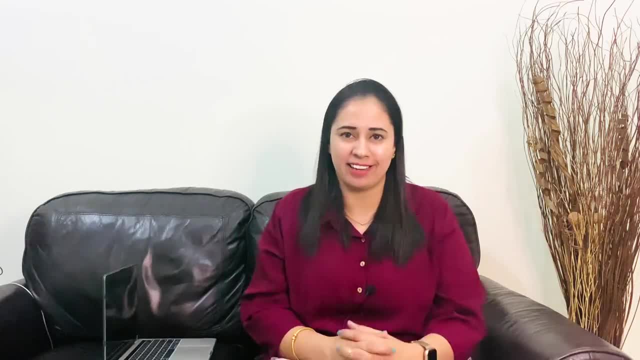 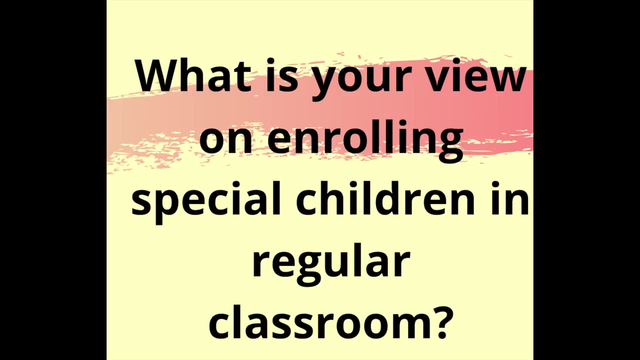 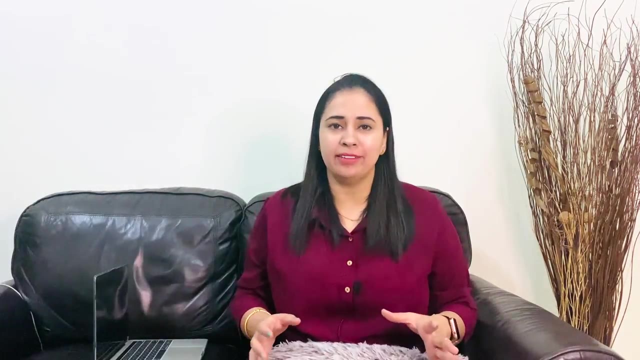 and they will really enjoy the lesson which is happening in the class. next question is: what do, what do you think about the special need children? do we have to enroll them in the regular classroom? so you justify your answer means why or why not. so you can say: see, it's totally depend on the type of disability. if the disability is physical and 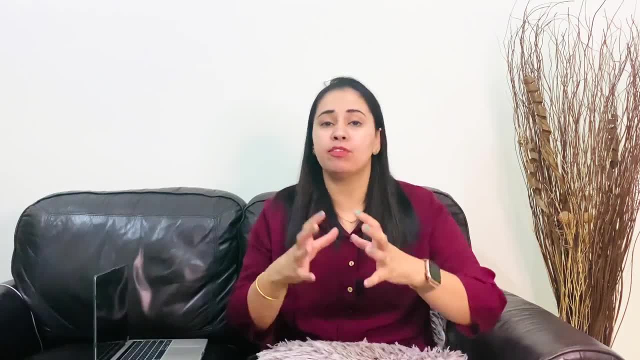 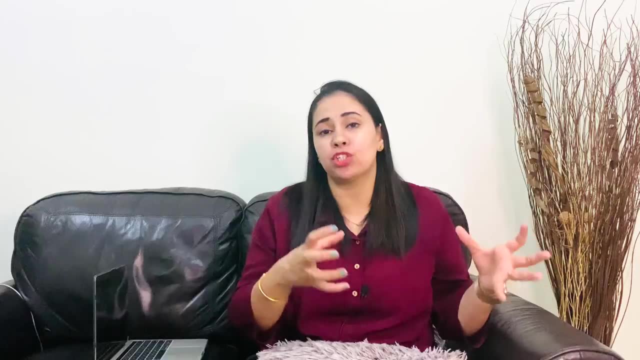 the child will able to cope up mentally in the class, then we do have to enroll them with the regular students in the regular classrooms. but if the student need some special help, some extra care where they can be involved, then we have to enroll them right away and the students will be able to. 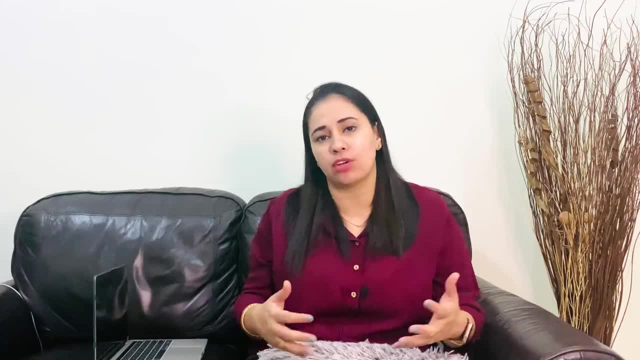 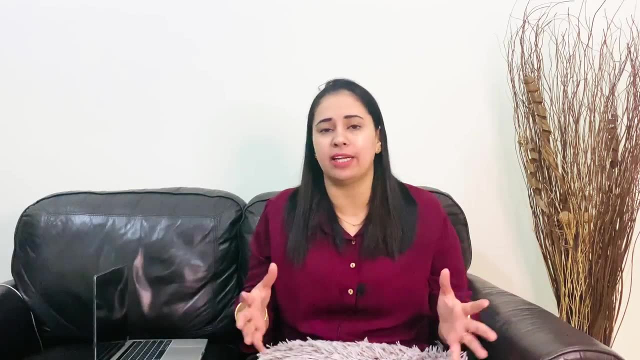 he will not feel lost and, if you know, a struggle to cope up with the normal classroom. so we need to take, we need to enroll them with the special classroom, like if the disability is with the eyes- they are not able to speak up. so in those kind of disability where they are not able to cope up with 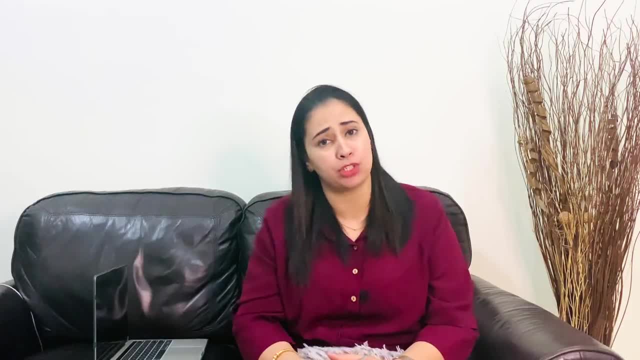 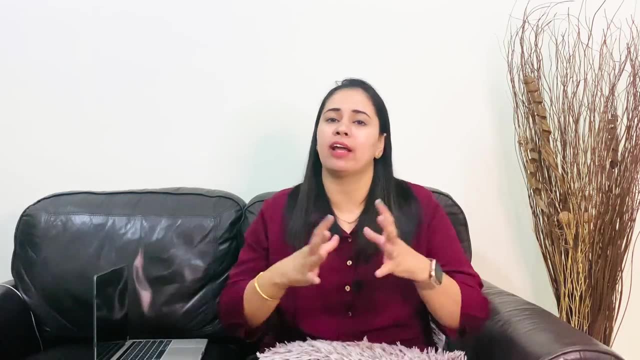 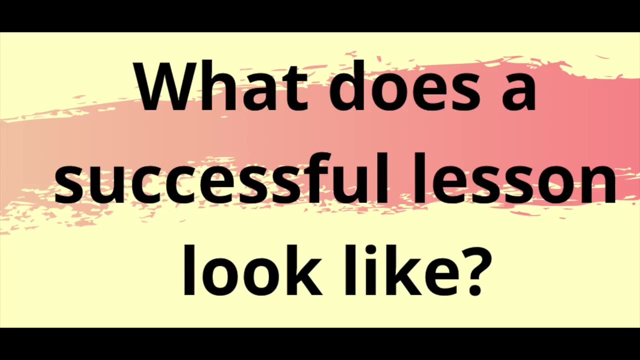 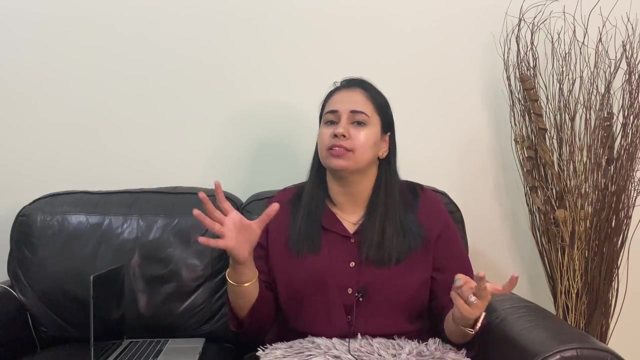 the regular classroom. that time we can enroll them in the special courses or the special classroom. otherwise, according to my view, we have to try at least to enroll them with the regular classrooms. question number five: tell me, according to your view, what the successful lesson look like, so you can say that see, according to me, two things make a lesson successful. the first thing is: 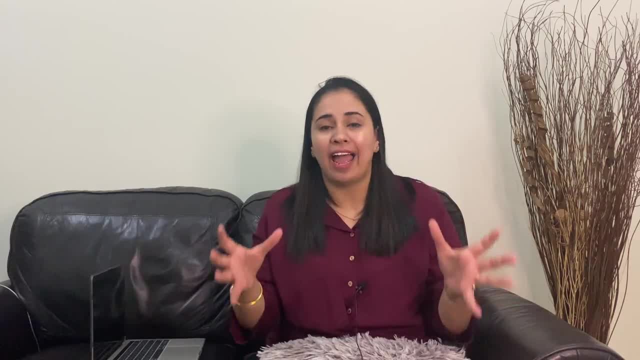 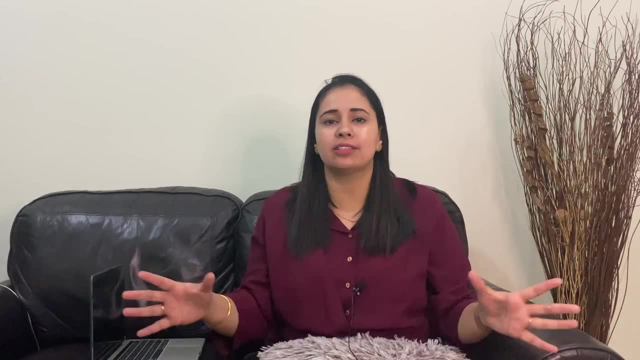 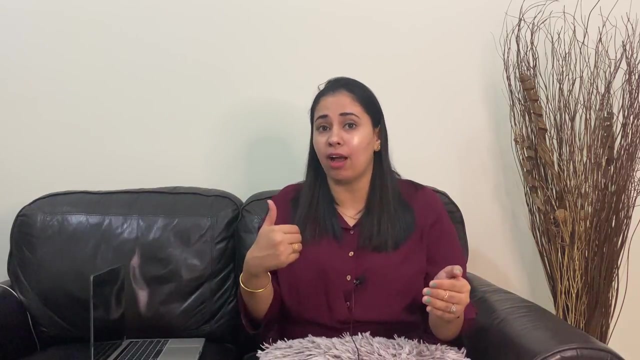 if i am able to bring the maximum interaction and the interest of the lesson, interest of the students in the lesson, if they will enjoy my lesson, so that is a successful criteria. the second thing is about the learning outcomes. if i am able to achieve my learning outcomes with the interest and with the, by making the